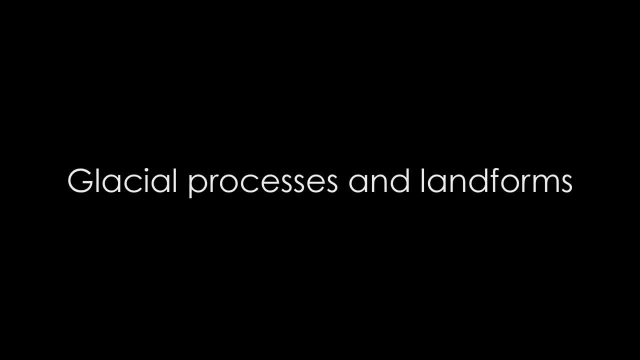 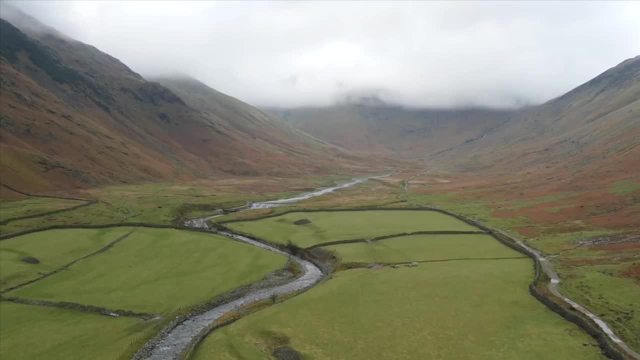 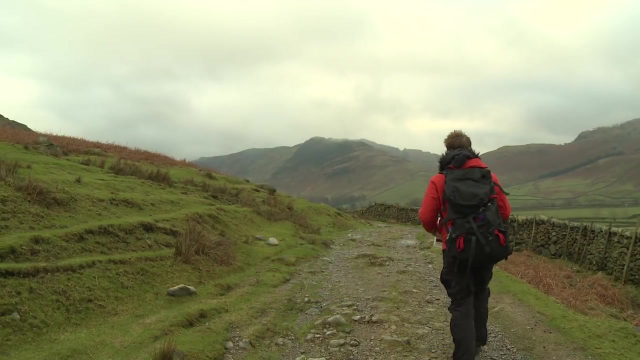 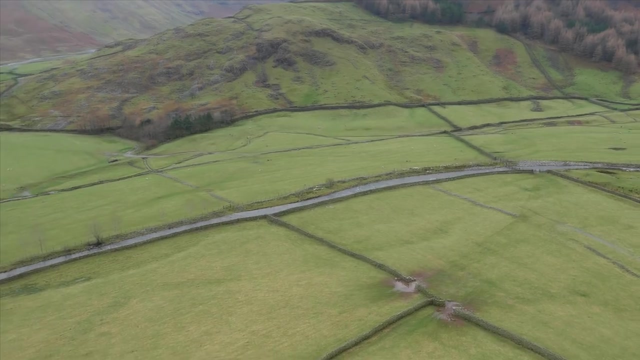 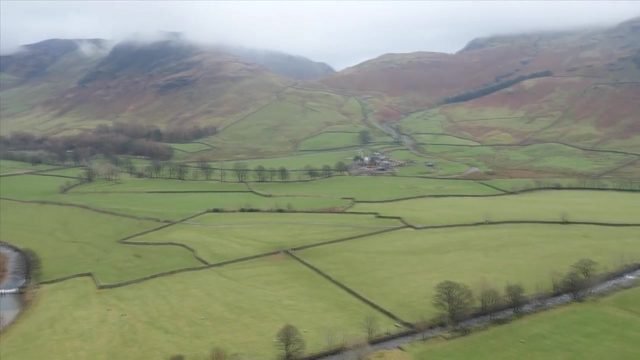 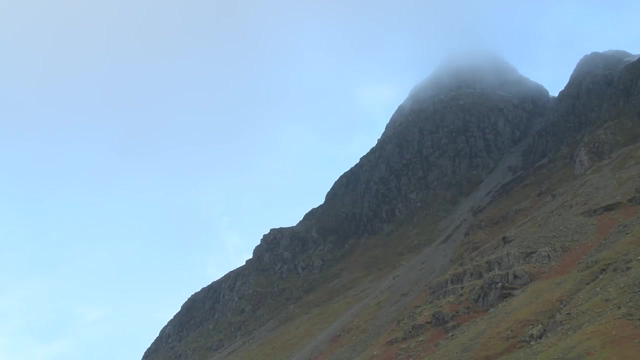 Today I'm glacier hunting here in the Lake District in England. Although it's hard to imagine, we once had glaciers here in the UK, Going back 18,000 years to the last ice age. these mountains were buried in ice and were perfect glacier-forming territory. 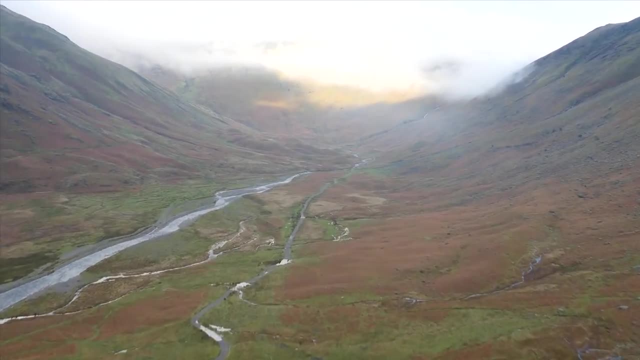 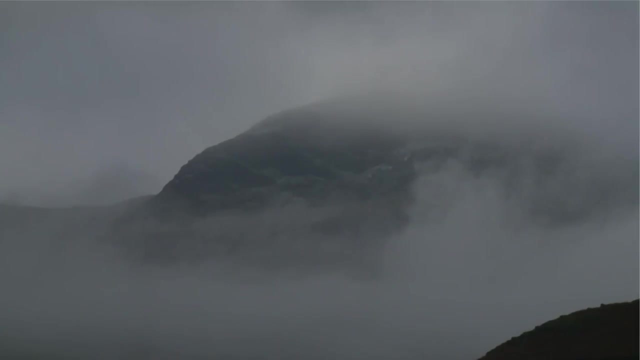 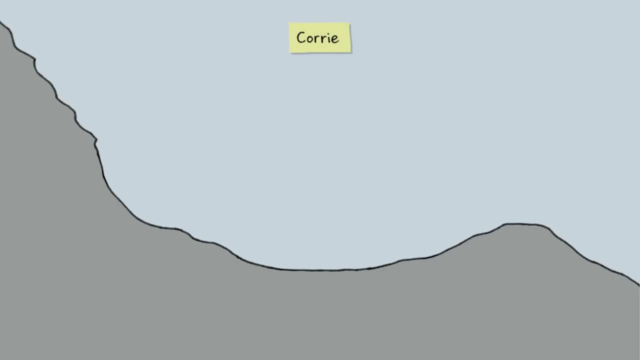 And it was these glaciers that radically transformed the landscape into what we see today. It was high up in the mountains where the glacier was born, in a corrie, or coombe as they're known in Wales. These corries were formed when snow collected year on year in hollows on the mountainside. 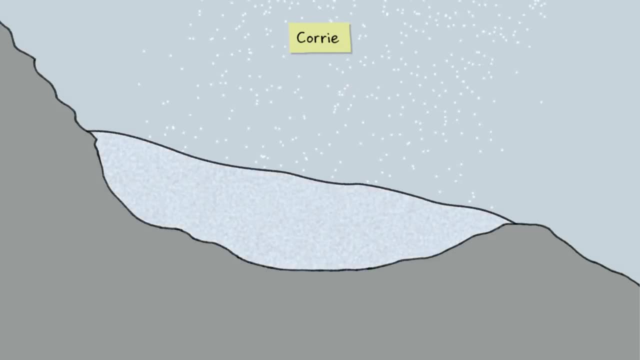 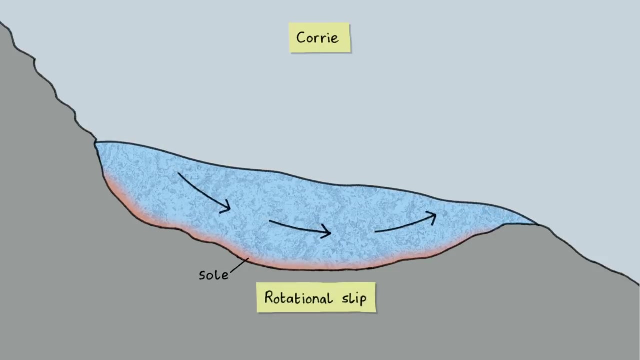 gradually forming incredibly strong, tightly packed ice. Once there was enough ice, it started to move, because the ice at the bottom, or soul of the glacier, melts under intense pressure from the weight of the ice above, allowing the ice to move in what's known as rotational slip. 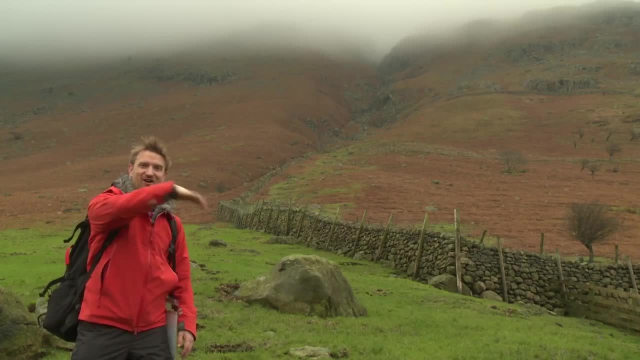 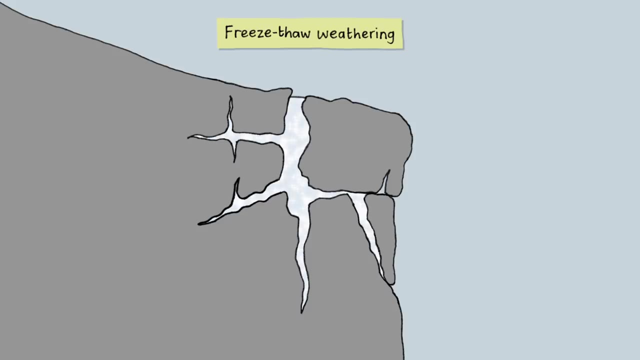 It's a bit like your bottom sliding down the back of a car. It's a bit like your car seat. Freeze, thaw weathering takes place above the glacier as ice thaws and then re-freezes inside cracks or fissures in the rock. 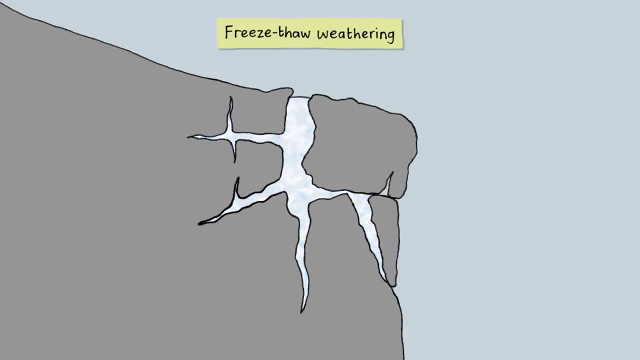 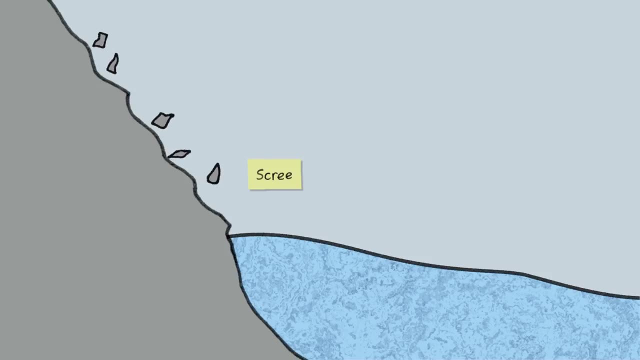 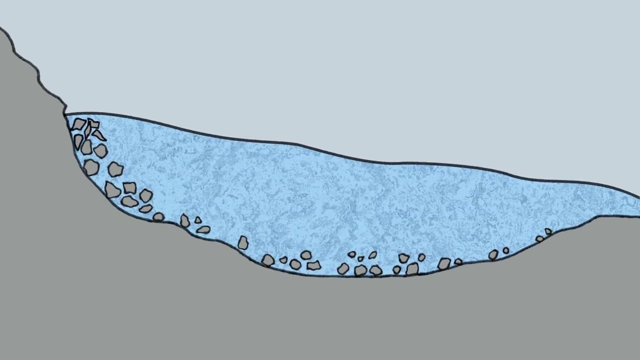 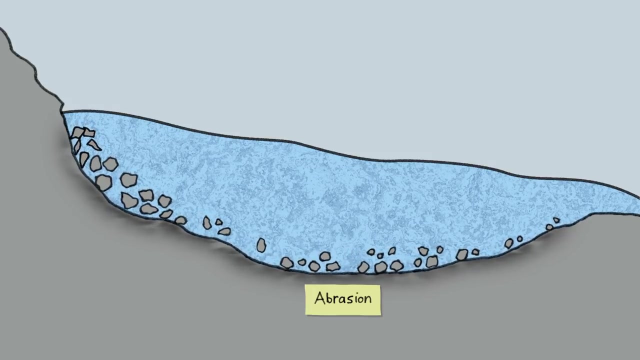 Each time water freezes, it expands, widening the crack a small amount. Eventually the rock will burst apart. Stone fragments, called scree, fall onto the glacier. These rocks join other debris picked up by the ice at the soul of the glacier. As the glacier moves, abrasion kicks in. as these stones scrape along the rock floor. 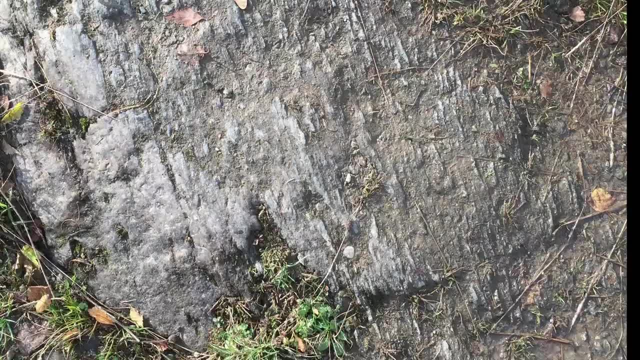 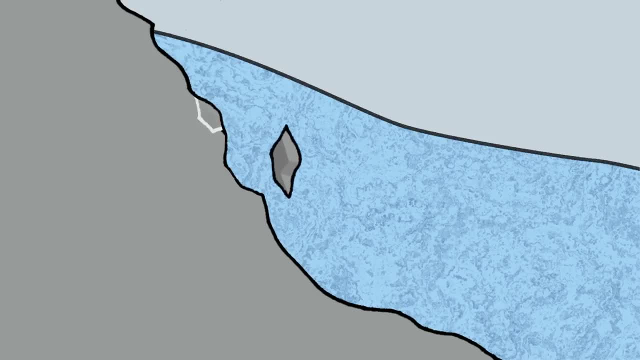 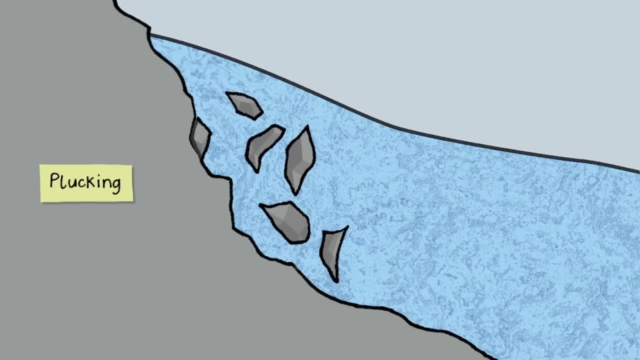 And you can see how these stones scoured the surface of the land like supercharged sandpaper, deepening and smoothing it Over time. by melting and re-freezing around a large rock, the ice simply lifts it away in a form of erosion known as plucking, to create the steep back walls and the armchair-shaped.